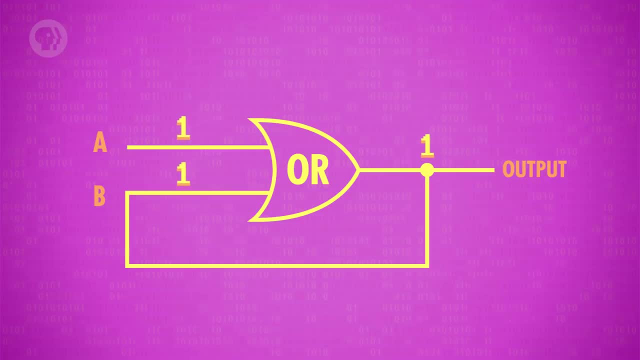 both of its inputs are now one. One OR one is still one, so there is no change in output. And if we flip input A back to zero, the OR gate still outputs one. So now we've got a circuit that records a one for us. 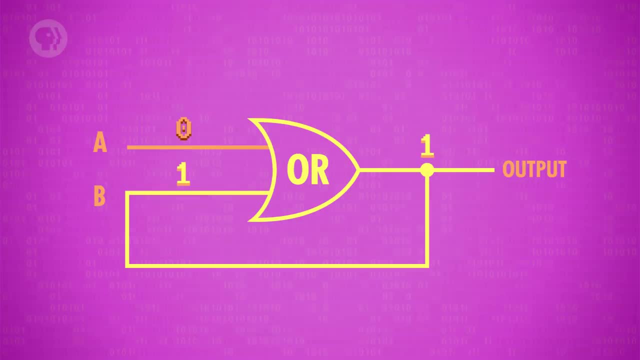 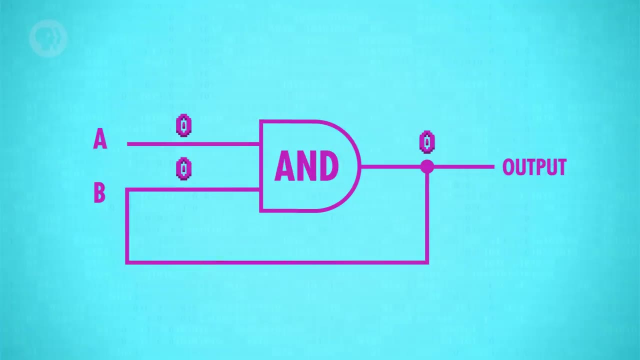 Except we've got a teensy, tiny problem. This change is permanent. No matter how hard we try, there's no way to get this circuit to flip back from a one to a zero. Now let's look at the same circuit, but with an AND gate instead. 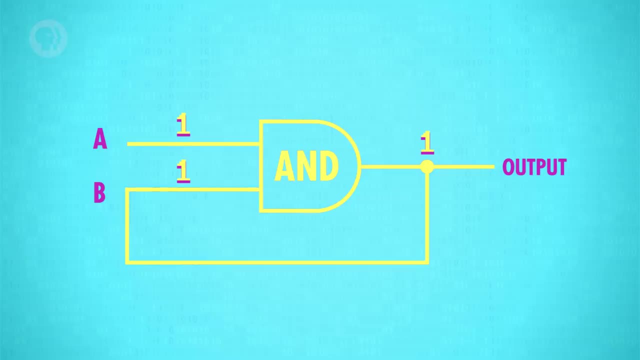 We'll start inputs A and B both at one. One AND one outputs one forever. But if we then flip input A to zero, because it's an AND gate, the output will go to zero. So this circuit records a zero. It's the opposite of our other circuit. 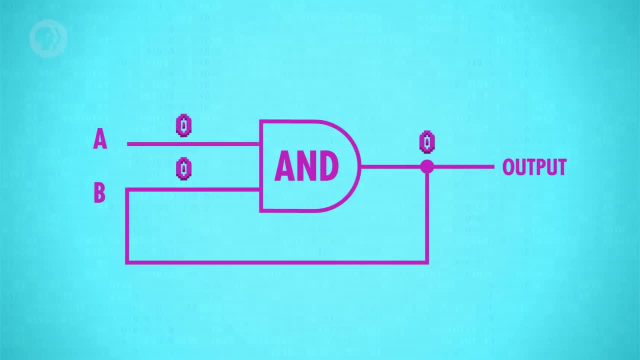 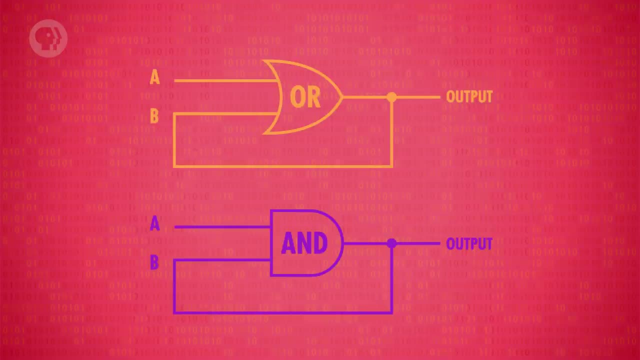 Like before, no matter what input we apply to input A afterwards, the circuit will always output zero. Now we've got the circuits that can record both zeros and ones. The key to making this a useful piece of memory is to combine our two circuits into what's. 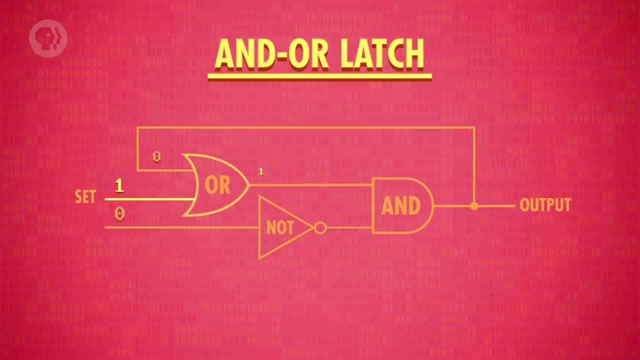 called the AND OR latch. It has two inputs: a set input, which sets the output to a one, and a reset input which resets the output to a zero. If set and reset are both zero, the circuit just outputs whatever was last put in it. 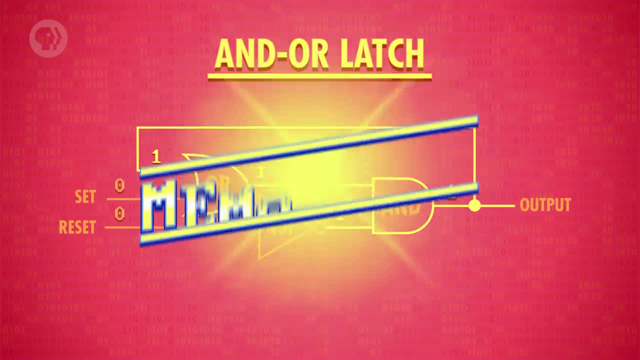 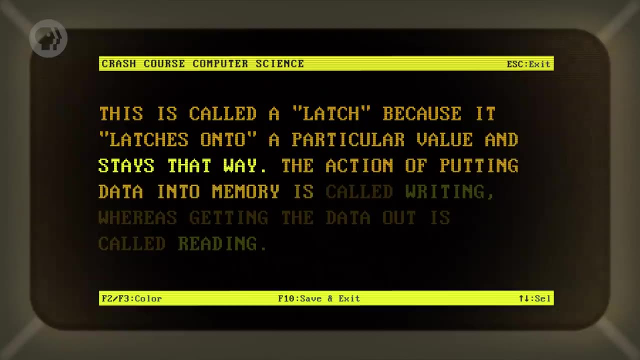 In other words, it remembers a single bit of information Memory. This is called a latch, because it latches onto a particular value and stays that way. The action of putting data into memory is called writing, whereas getting the data out is called reading. 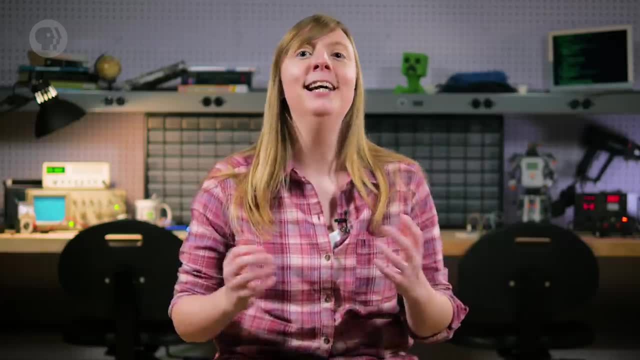 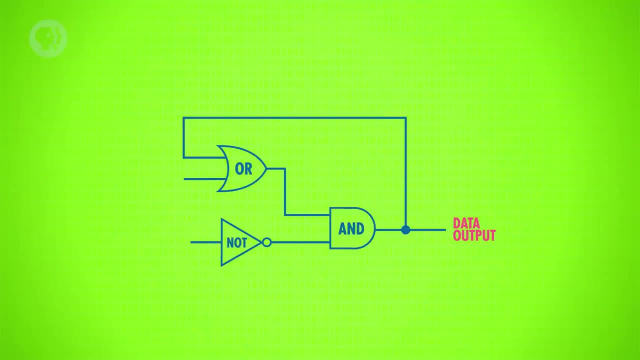 OK, so we've got a way to store a single bit of information- Great. Unfortunately, having two different wires for input, set and reset is a bit confusing. To make this a little easier to use, we really want a single wire to input data that we 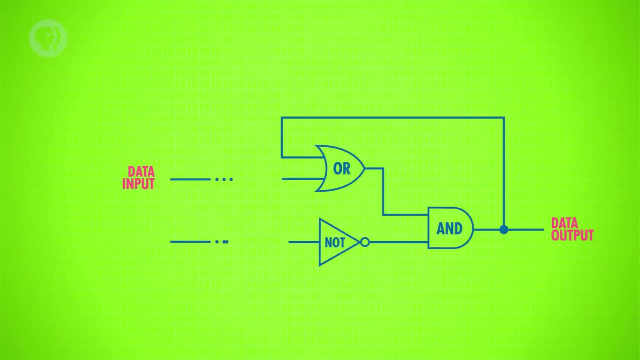 can set to either zero or one to store the value. Additionally, we're going to need a wire that enables the memory on the input, So we're going to need a single wire to input data that we can set to either zero or one to store the value. 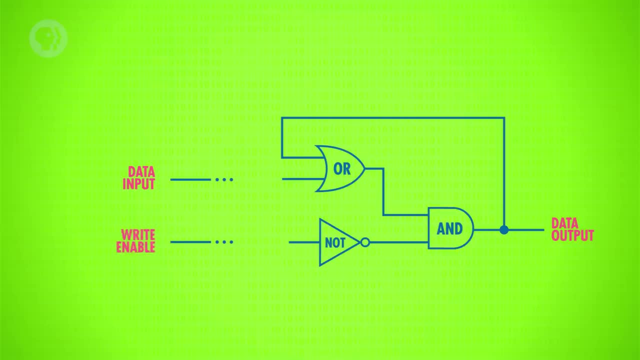 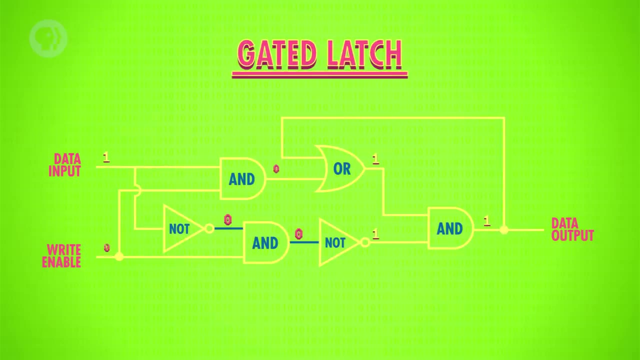 This one is either to be available for writing or locked down, which is called the write-enable line. By adding a few extra logic gates, we can build this circuit, which is called a gated latch, since the gate can be opened or closed. 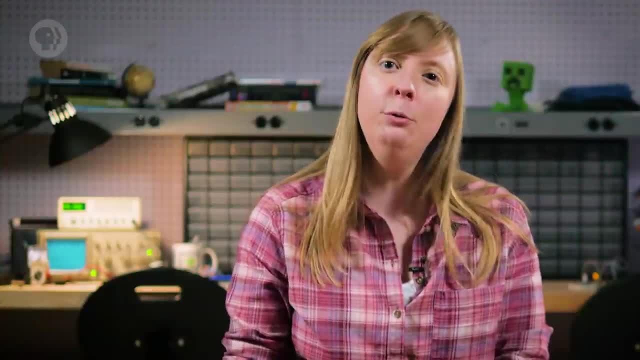 Now this circuit is starting to get a little complicated. We don't want to have to deal with all the individual logic gates so, as before, we're going to bump up a level of abstraction and put our whole gated latch circuit in a box. 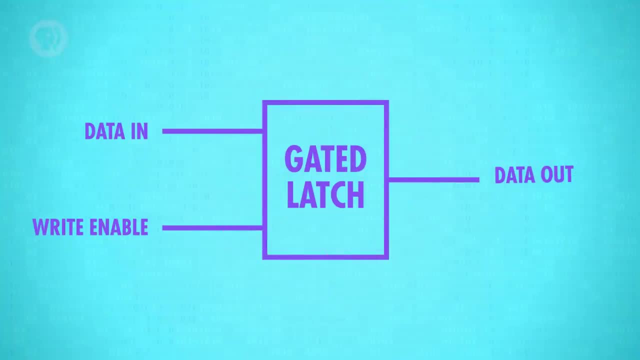 A box that stores one bit. Let's test out our new component. Let's start everything at zero. If we toggle the data wire from zero to one or one to zero, then the data will be stored in memory. Nothing happens. The output stays at zero. 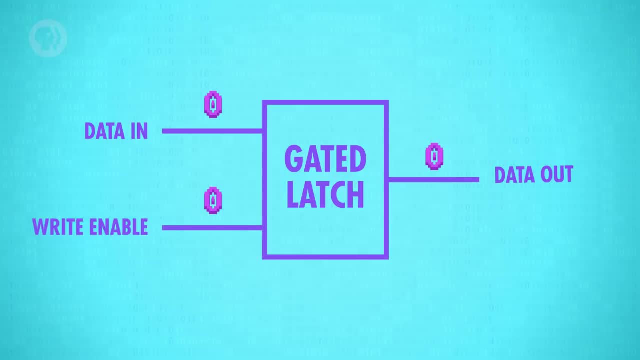 That's because the write-enable wire is off, which prevents any change to the memory. So we need to open the gate by turning the write-enable wire to one. Now we can put a one on the data line to save the value to our latch. 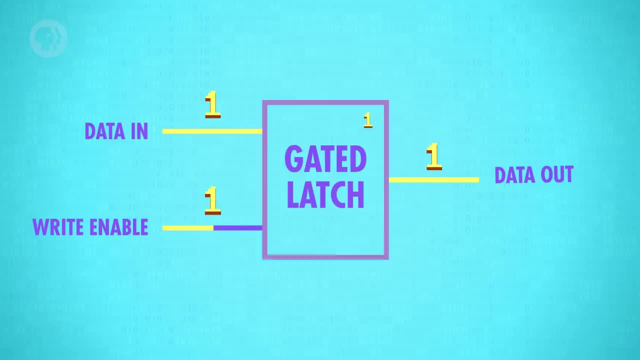 Notice how the output is now one. Success: We can turn off the enable line and the output stays as one. Once again, we can toggle the value on the data line all we want, but the output will stay the same. The value is saved in memory. 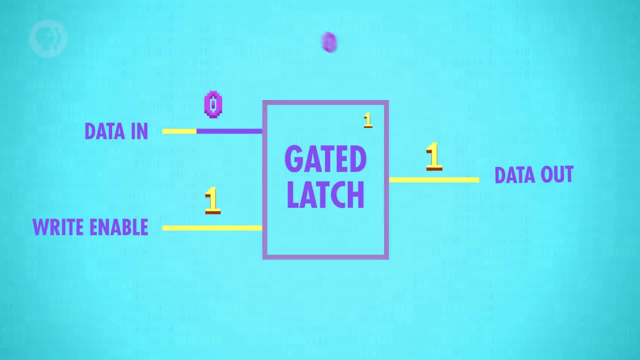 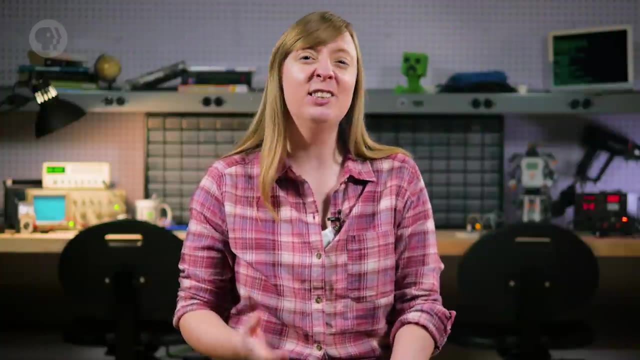 Now let's turn the enable line on again And use our data line to set the latch to zero. Done Enable line off, the output is zero and it works. Now, of course, computer memory that only stores one bit of information isn't very useful. 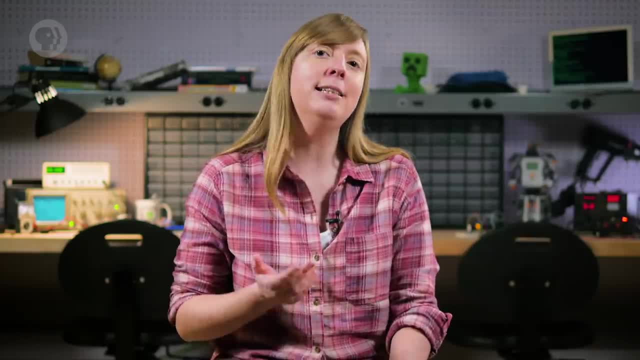 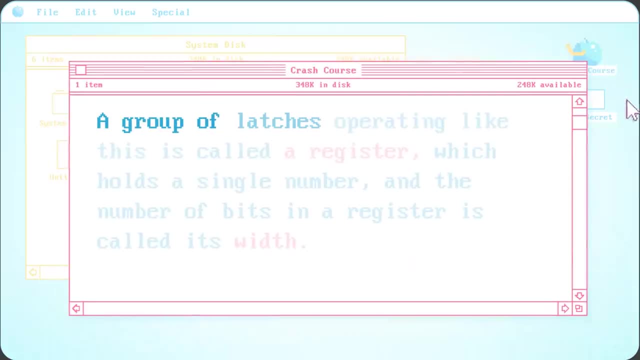 Definitely not enough to run Frogger or anything really. But we're not limited to using only one latch. If we put 8 latches side by side, we can store 8 bits of information like an 8-bit number. A group of latches operating like this is called a register, which holds a single number. 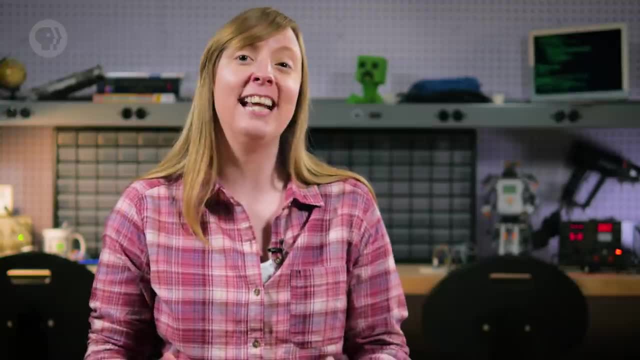 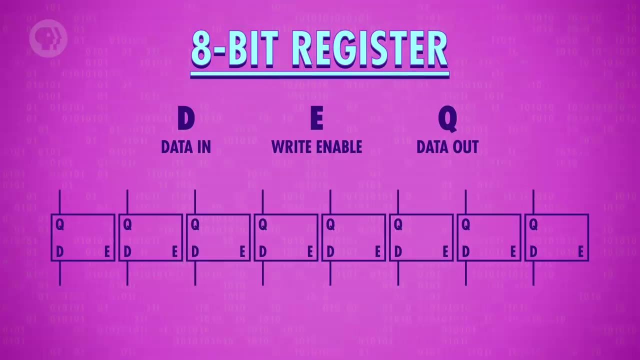 And the number of bits in a register is called its width. Many computers had 8-bit registers, then 16,, 32, and today many computers have registers that are 64 bits wide. To write to our register we first have to enable all of the latches. 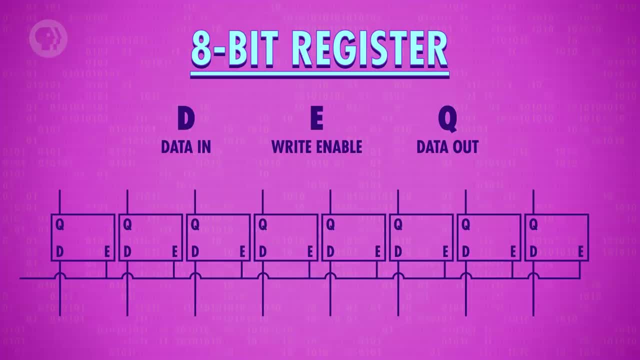 We can do this with a single wire that connects to all of their enable inputs, which we set to 1. We then send our data in using the 8 data wires and then set the enable back to zero And the 8-bit value is now saved in memory. 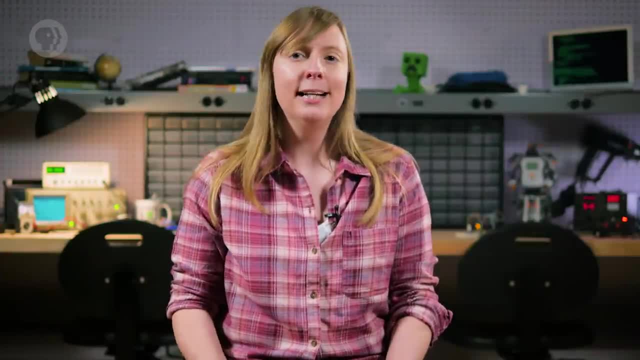 Putting latches side by side works OK for a smallish number of bits. A 64-bit register would need 64 wires running to the 8-bit register, And that's it. Thanks for watching. If you liked this video, be sure to give it a thumbs up and subscribe to our channel. 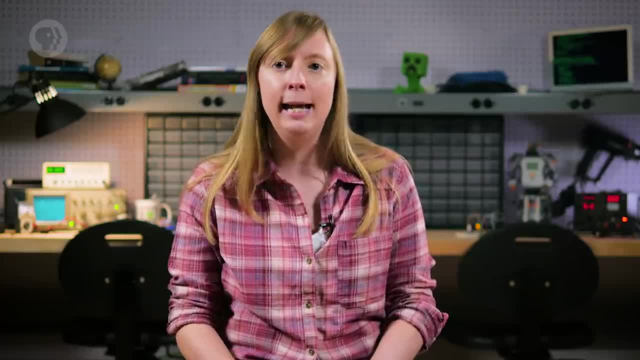 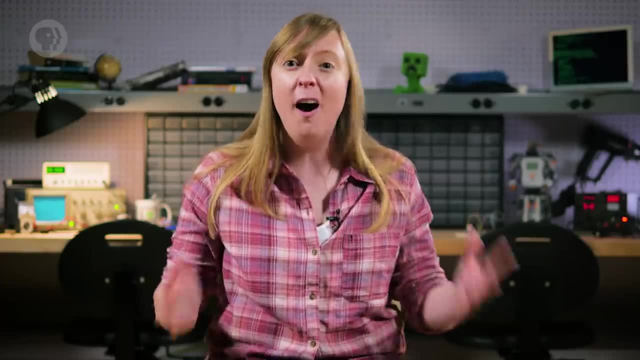 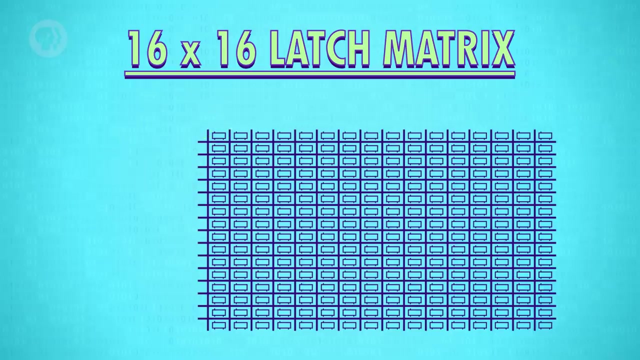 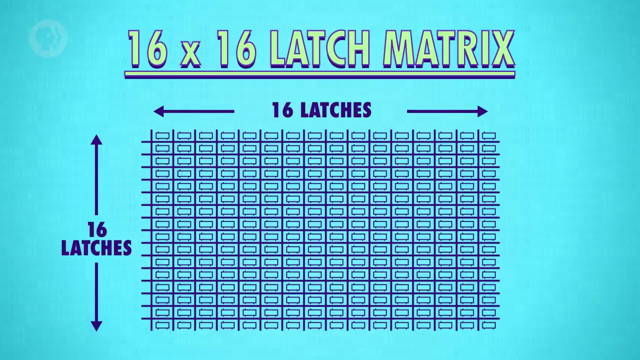 if you want to see more videos like this one, And don't forget to turn on your notifications so you don't miss out on any of our new videos. We'll see you in the next video. Bye for now. Let's zoom in and see how this works. 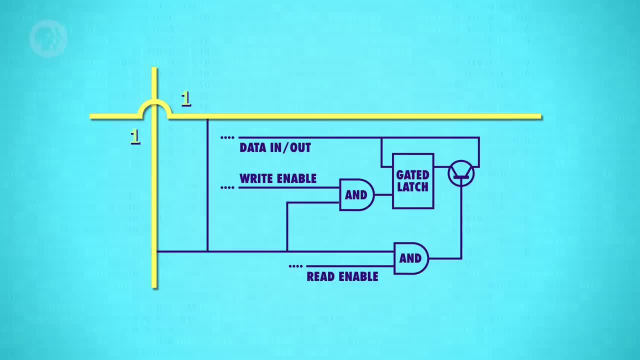 We only want the latch at the intersection of the two active wires to be enabled, But all of the other latches should stay disabled. For this we can use our trusty AND gate. The AND gate will output a 1 only if the row AND the column wires are both 1.. 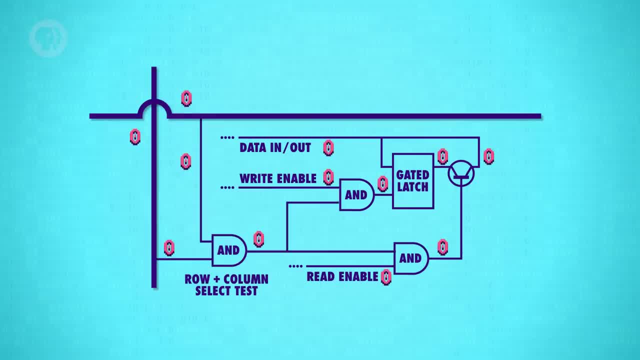 So we can use this signal to uniquely select a single latch. This row and column setup connects all of our latches with a single shared write-enable wire. In order for a latch to become write-enabled, the row wire, the column wire and the write-enable. 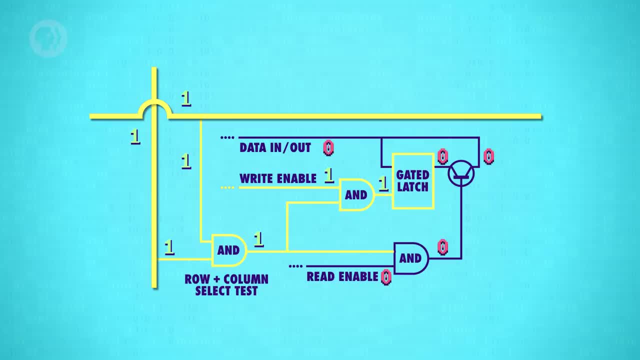 wire must all be 1.. That should only ever be true for one single latch at any given time. This means we can use a single shared wire for data, because only one latch will ever be write-enabled, Only one will ever save the data. 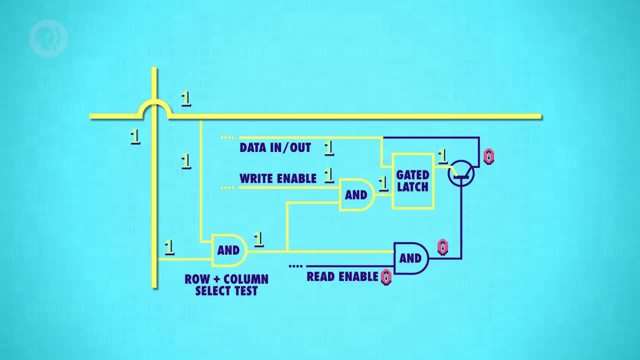 The rest of the latches will simply ignore values on the data wire because they are not write-enabled. We can use the same trick with a read-enabled wire to read the data later. to get the data out of one specific latch, This means in total, for 256 bits of memory. we only need 35 wires. 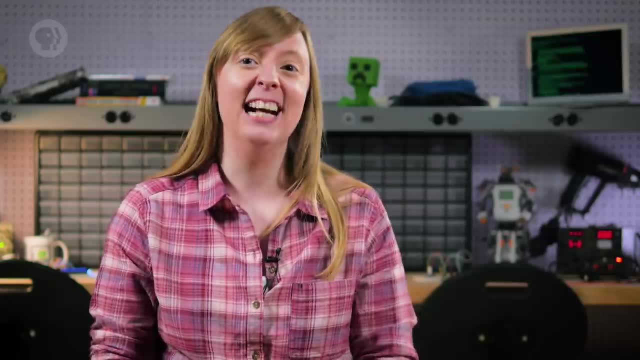 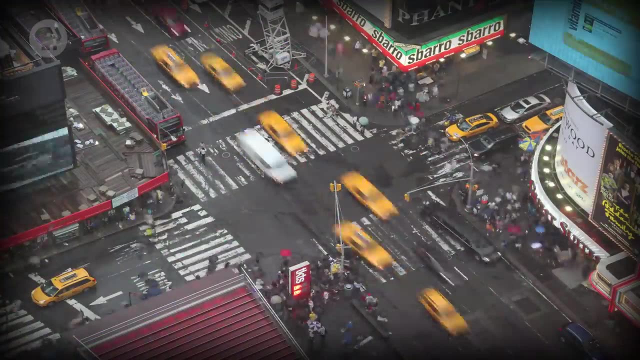 One data wire, one write-enabled wire, One read-enabled wire And 16 rows and columns for the selection. That's significant wire savings, But we need a way to uniquely specify each intersection. We can think of this like a city where you might want to meet someone at 12th Avenue. 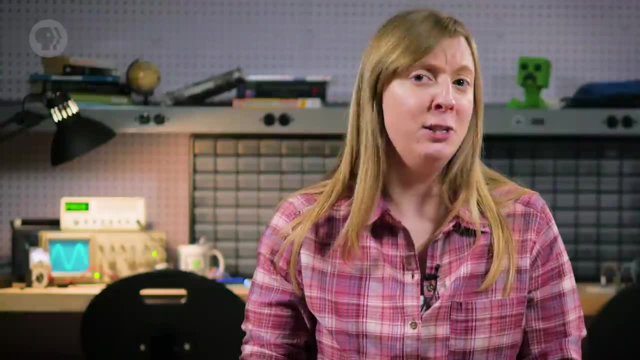 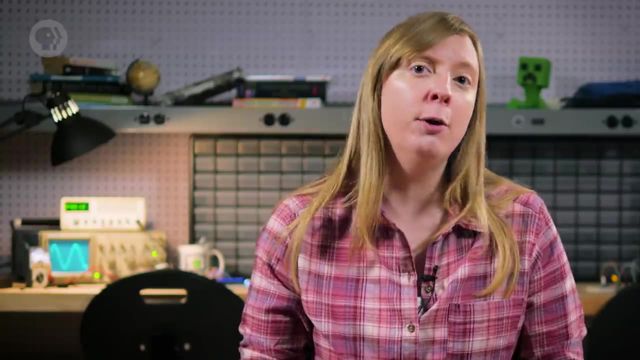 and 8th Street. That's an address that defines an intersection. The latch we just saved our 1-bit into has an address of row 12 and column 8.. Since there is a maximum of 16 rows, we store the row address in a 4-bit number. 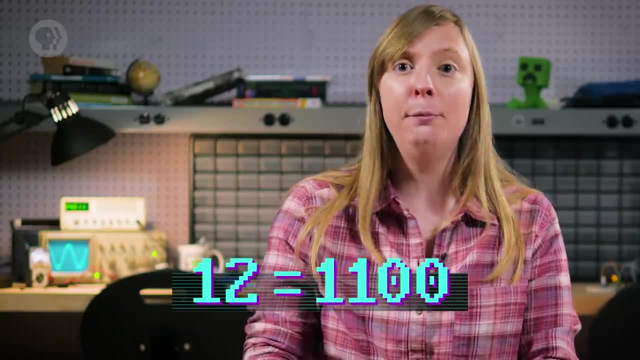 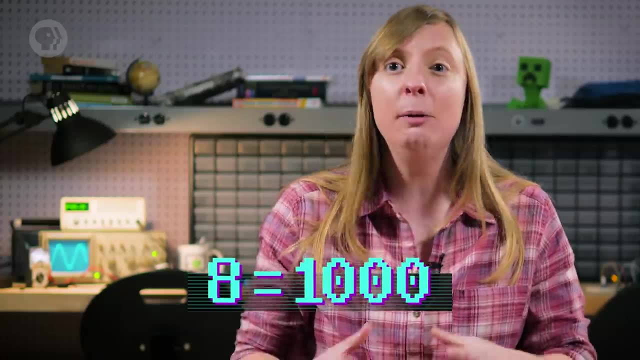 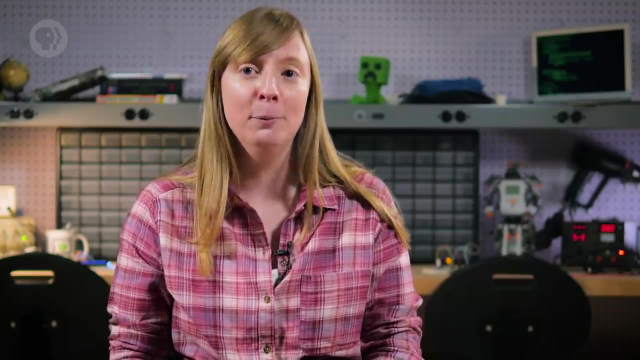 12 is 1100 in binary. We can do the same for the column address. 8 is 1000 in binary. So the address for the particular latch we just used can be written as 11001000.. To convert from an address into something that selects the right row or column, we need: 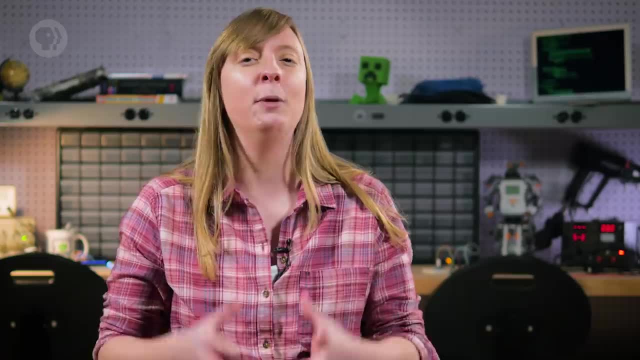 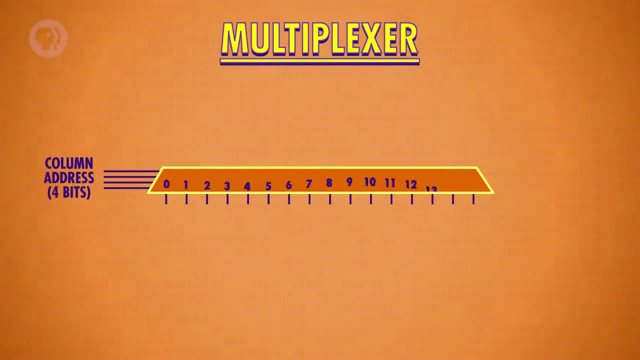 a special component called a multiplexer, which is a computer component with a pretty cool name, at least compared to the ALU. Multiplexers come in all different sizes, But because we have 16 rows, we need a 1-16 multiplexer. 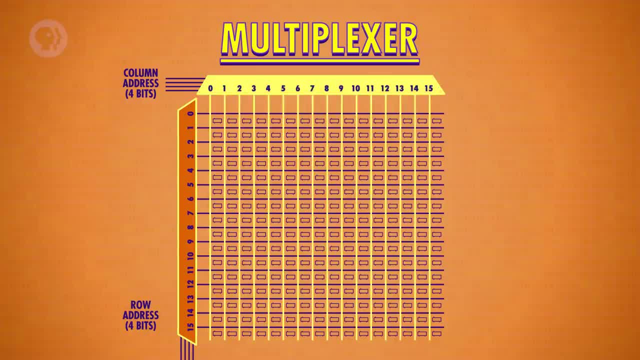 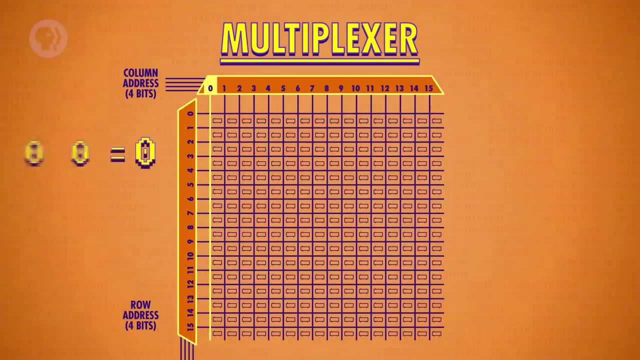 It works like this: We feed it a 4-bit number and it connects the input line to a corresponding output line. So if we pass in 0000, it will select the very first column for us. If we pass in 0001, the next column is selected, and so on. 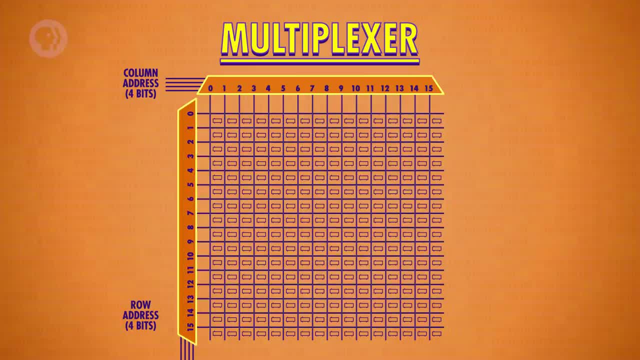 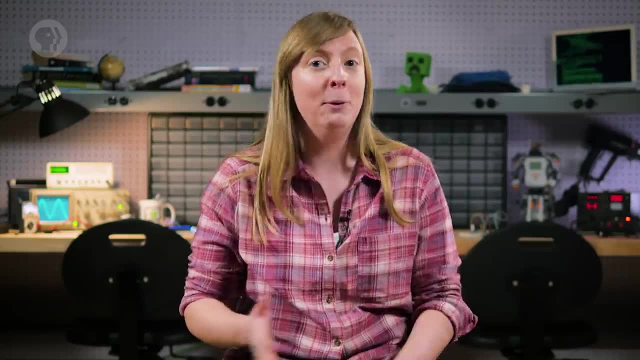 We need one multiplexer to handle our rows and another multiplexer to handle the columns. OK, it's starting to get complicated again, so let's make our 256-bit memory its own component. Once again, a new level of abstraction. 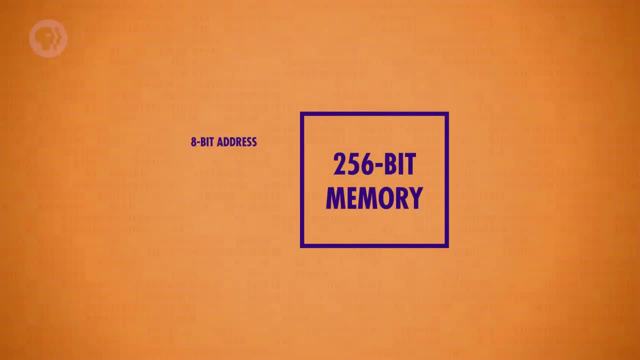 It takes an 8-bit address for input: the 4 bits for the column and 4 for the row. We also need write and read enable wires And finally, we need just one data wire which can be used to read or write data. 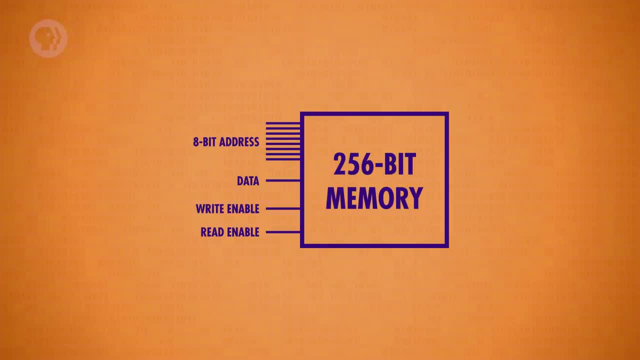 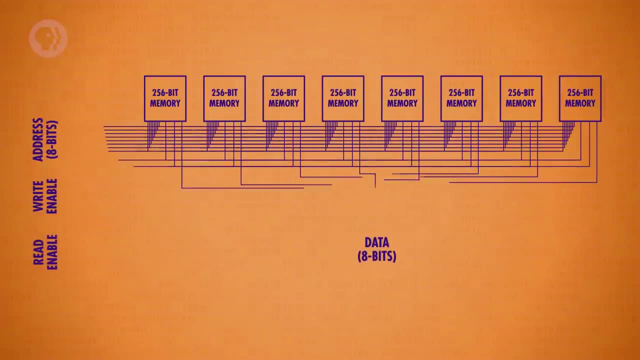 Unfortunately, even 256 bits of memory isn't enough to run much of anything, so we need to scale up even more. We're going to put them in a row, just like with the registers. We'll make a row of 8 of them so we can store an 8-bit number, also known as a byte. 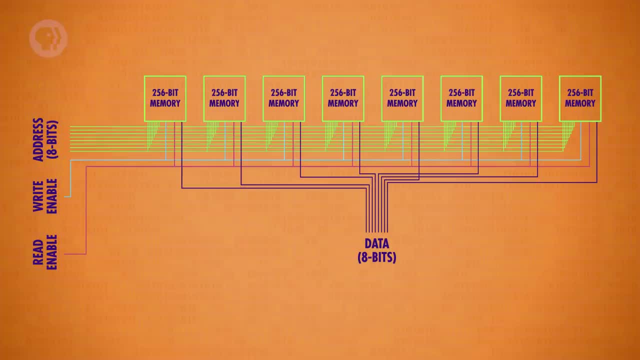 To do this, we feed the exact same address into all 8 of our 256-bit memory components at the same time, And each one saves one bit of the number. That means the component we just made can store 256 bytes at 256 different addresses. 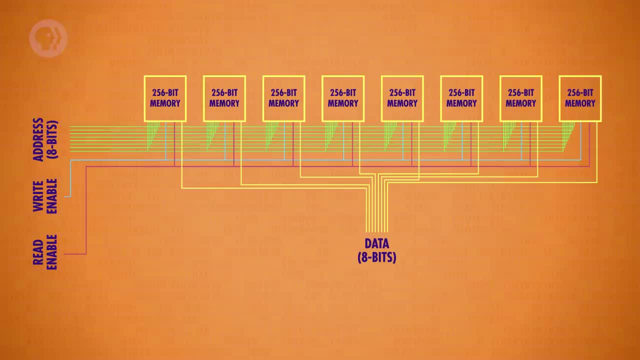 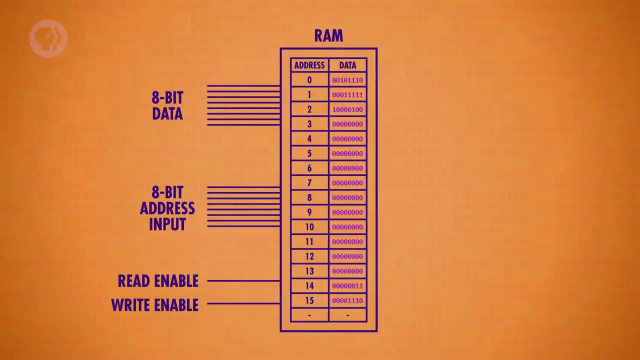 Again, to keep things simple, we want to leave behind this inner complexity. Instead of thinking of this as a series of individual memory modules and circuits, we'll think of it as a uniform bank of addressable memory. We have 256 addresses. 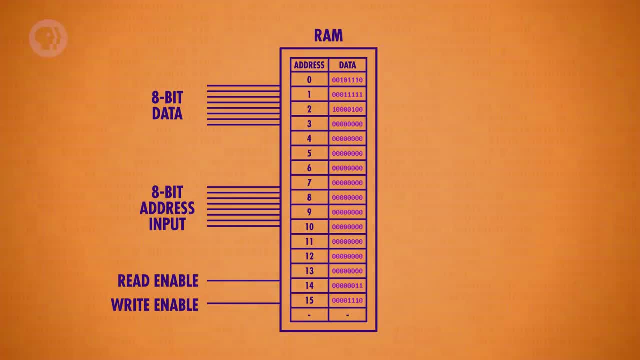 And at each address we'll have 256 addresses. And at each address we'll have 256 addresses We can read or write an 8-bit value. We're going to use this memory component next episode when we build our CPU. 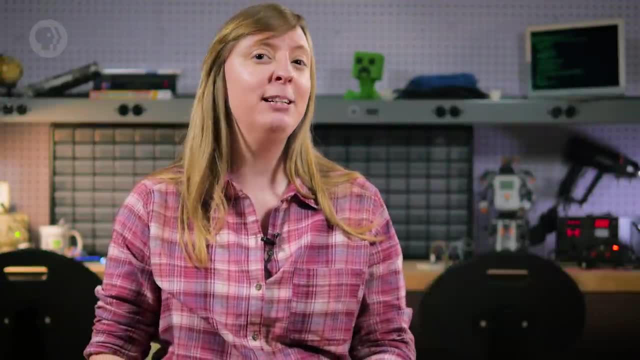 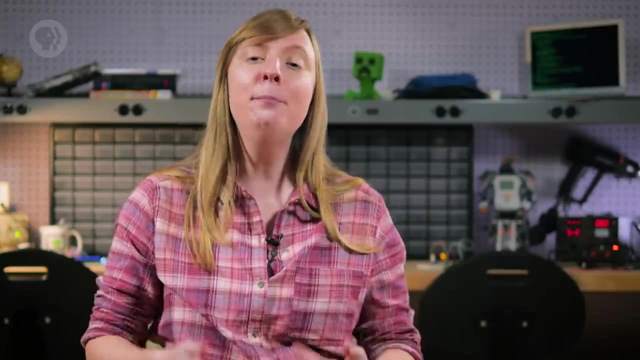 The way that modern computers scale to megabytes and gigabytes of memory is by doing the same thing we've been doing here: Keep packaging up little bundles of memory into larger and larger and larger arrangements. And as the number of memory locations grow, our addresses have to grow as well. 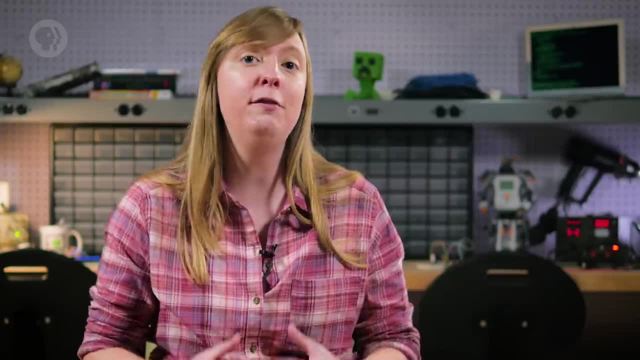 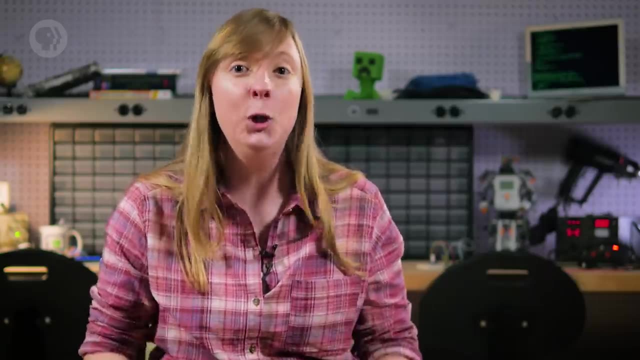 8 bits hold enough numbers to provide addresses for 256 bytes of our memory, But that's all. To address a gigabyte or a billion bytes of memory, we need to have a number of addresses. We need 32-bit addresses. 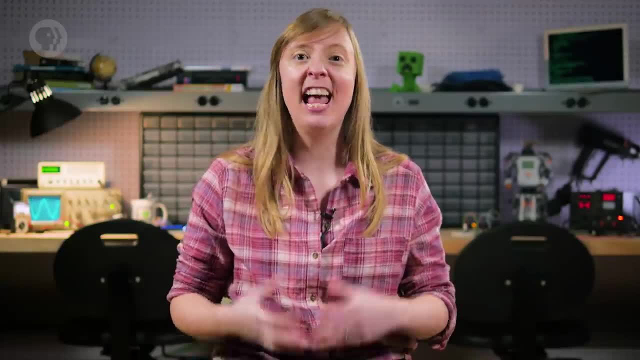 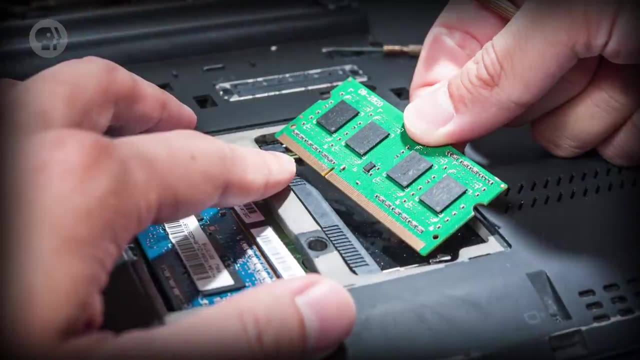 An important property of this memory is that we can access any memory location at any time and in a random order. For this reason, it's called Random Access Memory, or RAM. When you hear people talking about how much RAM a computer has, that's the computer's. 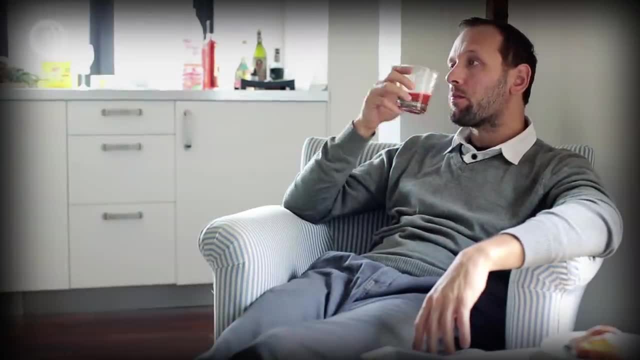 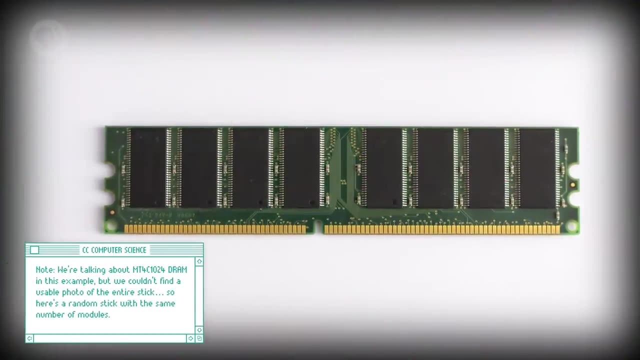 memory RAM is like a human's short-term or working memory, where you keep track of things going on right now, like whether or not you had lunch or paid your phone bill. Here's an actual stick of RAM with 8 memory modules soldered onto the board.